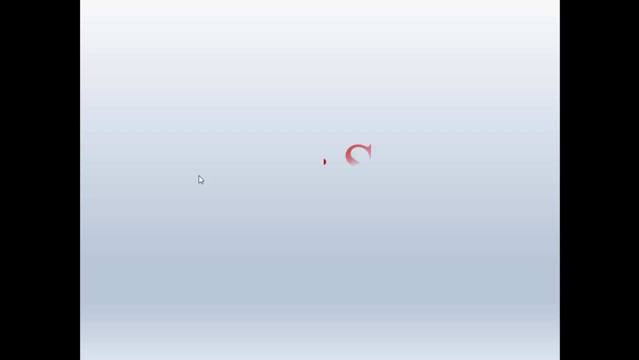 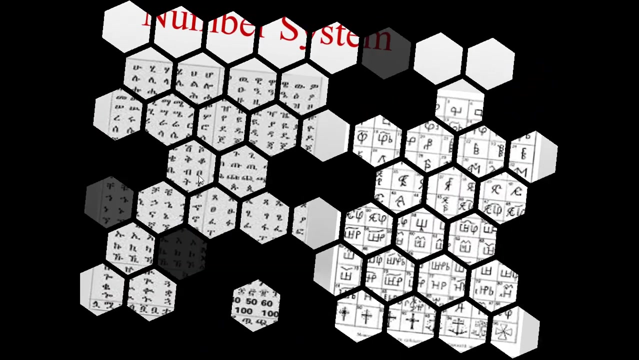 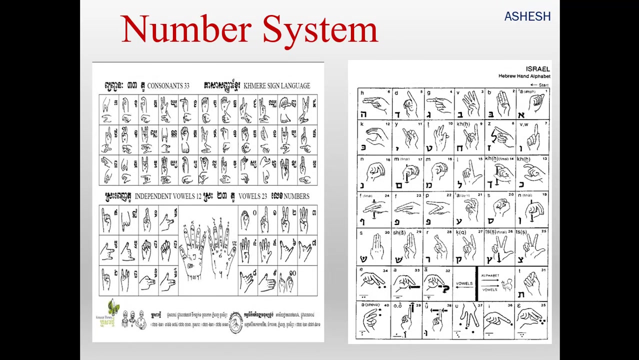 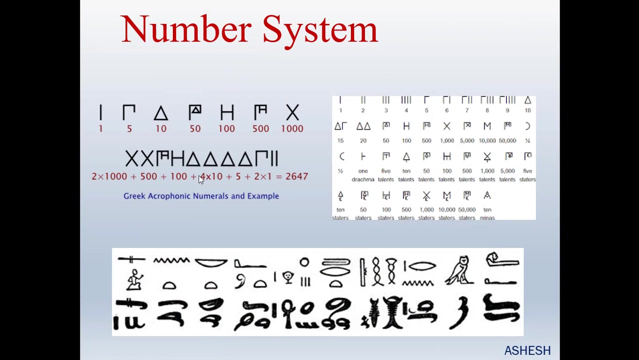 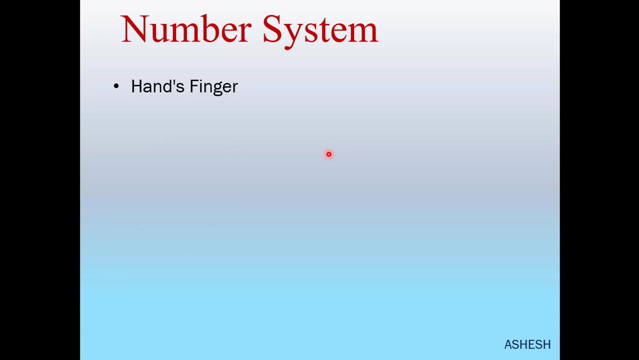 Hello, welcome to my channel, ICT blog. Today we'll know about the positional and non positional numbers of the number system. Here we see some ancient symbols. In the pictures we see some hands by showing some symbols. Here also some symbols, or count their numbers by head's finger, such as that or pebbles, or note of the rope, or 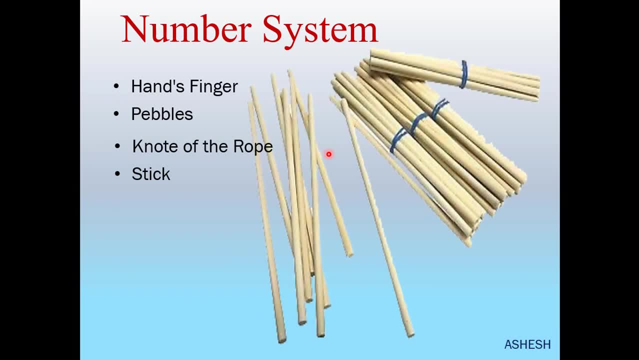 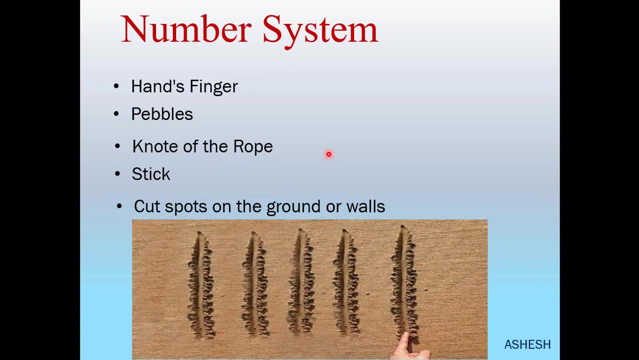 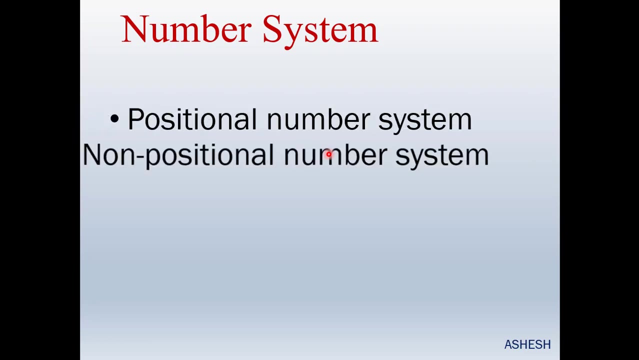 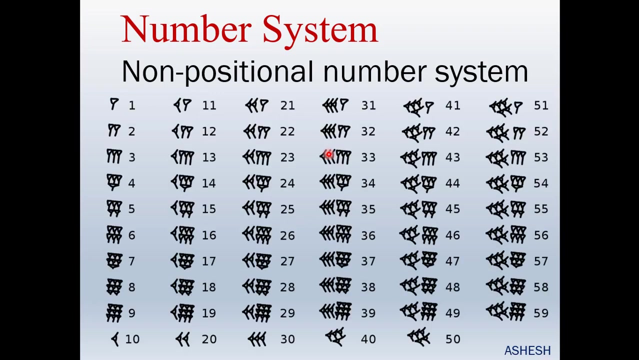 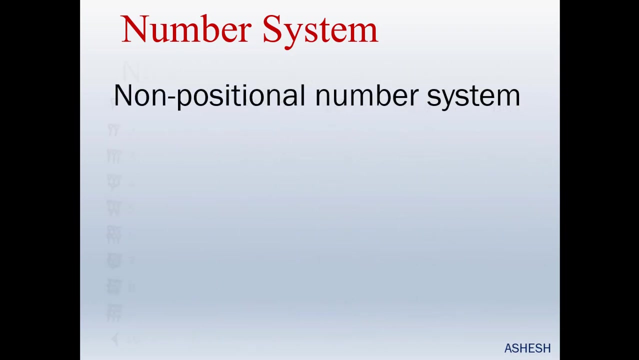 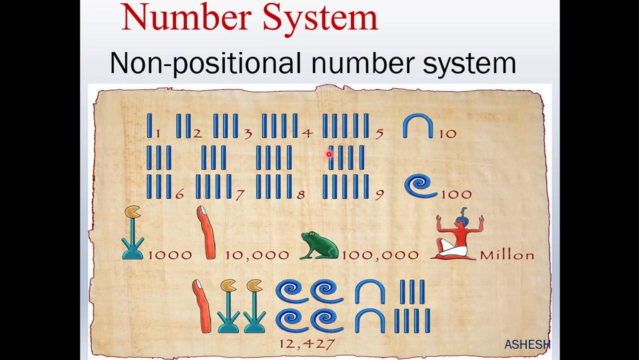 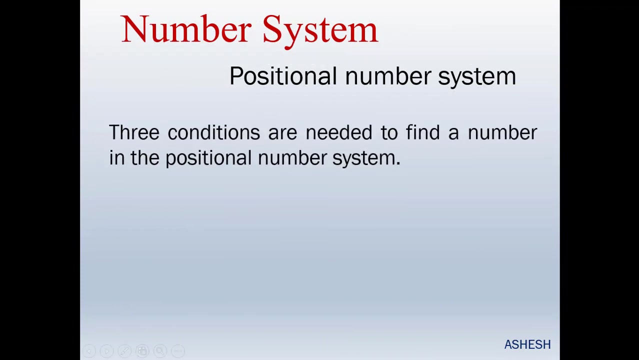 by sticks or by cut spots of the ground or wall. Here. positional number systems and non- positional number system. picture shows non- positional numbers. This also. this also shows non- positional number systems. Positional number system: three conditions are needed to find a number in the positional. 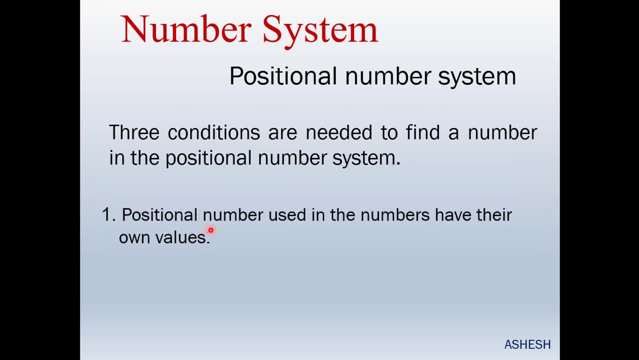 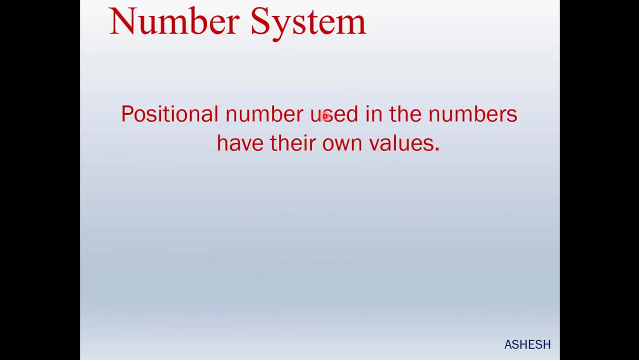 number system. One: positional number used in the number system Have their own values. two: the base of the number systems. three, the positional or local value of the numbers used in the positional numbers. Positional number used in the numbers have their own values, such as each number has. 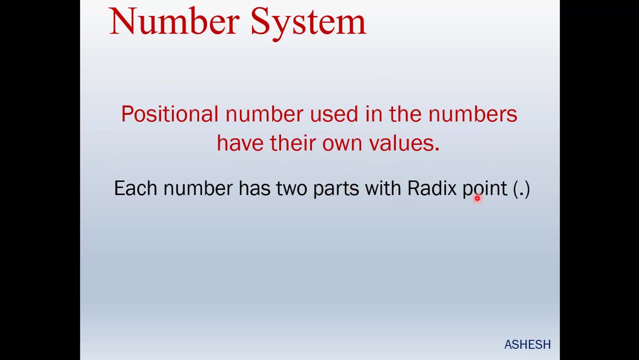 two parts with radix point. Let's see First one is integer and second part is fraction. Here we see some numbers: two, five, three, seven, six. Two, five, three, seven, six is integer number. and after point, after point, or radix point. 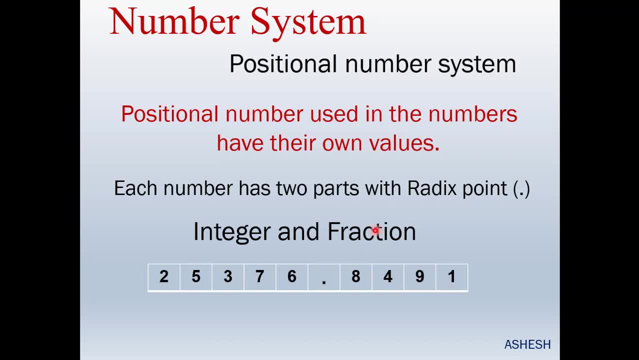 eight, four, nine, one is fraction, So that point is called fraction. So that point is called fraction. So that point is called fraction. Now say- you already know it right- Redix point. then we can say: before the radix point is integer and after the 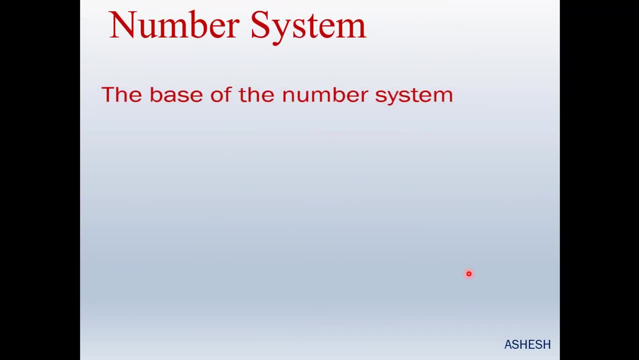 radix point is fraction. Second one: the base of the number systems. We know that decimal or tan-based number systems. Decimal number has product as number. if you can still search So far we have come ten based number systems, binary, or two base number systems. we know that binary. 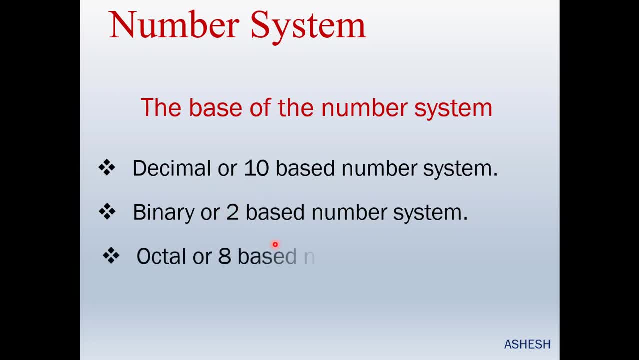 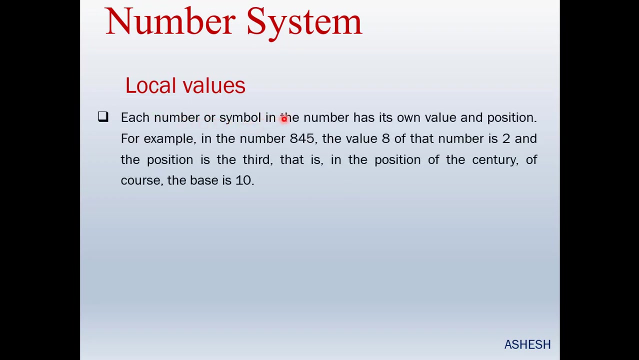 number has two base number systems, three octal or eight base number systems. we also know that octal number has eight based number systems and also hexadecimal or 16 base number system. local values. each number or symbol in the number has its own values and position. for example, in the number 8, 4, 5, the value 8 of the 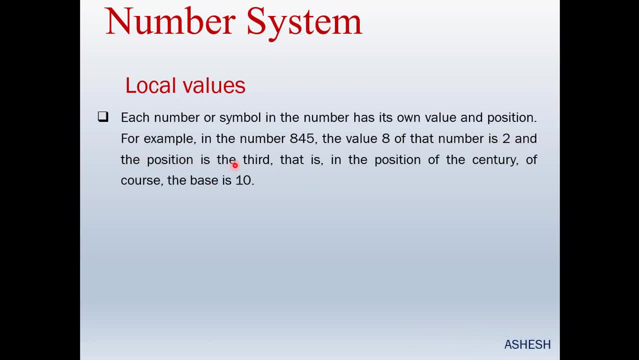 number is 2 and the position is 1: 1st, 2nd, 3rd- in the position of the system, century. of course the base is 10, so we see that 8 is a position of the century and the value of the number is 2, again 8 in the position of century and the value 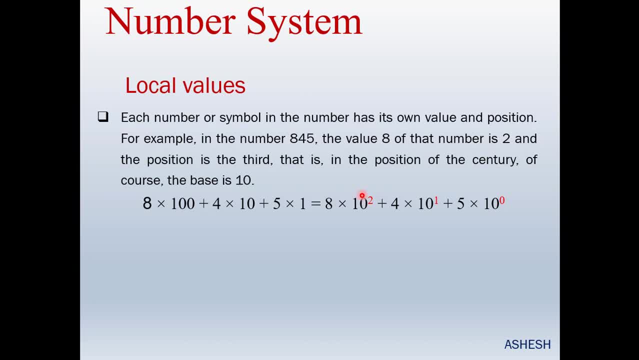 of 8 number is 2. again, there's another number: 485, has above three digits, above three, Pamamenko's home, Uhh is it? but it means another number due to daily Indoor 보기자는, Greed, location of the dановiat. that is the number or is in the 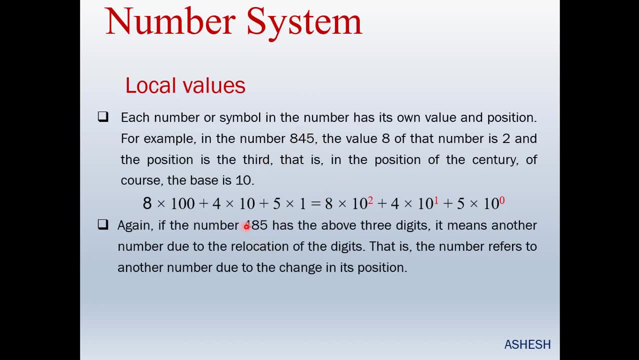 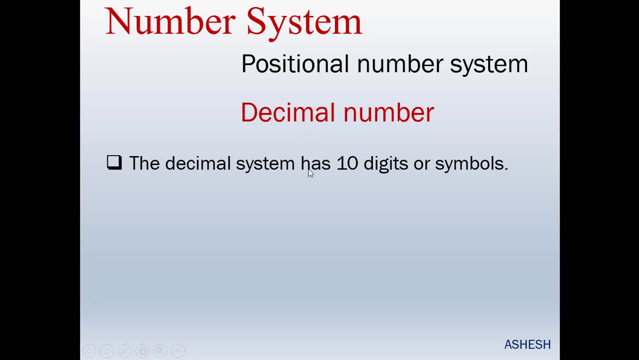 refers to another number, to another number, due to that change in its positions, then the number system consists of the number of the product, of two product, that is, the two are the own values of the symbols used in the numbers and the local value, now decimal number. the decimal number system has 10 digit or symbols. 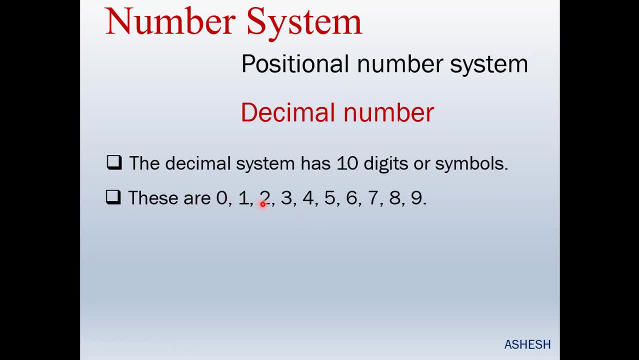 these are. these are 0, 1, 2, 3, 4, 5, 6, 7, 8, 9, but not 10. the maximum value of the digit in the decimal number is 9 and lowest number is 0 in decimal number system, base of 10. decimal number system is used in our daily life. 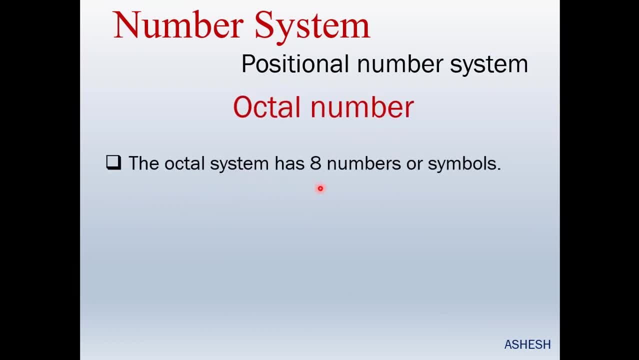 octal number system has eight numbers or symbols. these are zero, one, two, three, four, five, six, seven. but remember, not eight, not eight, only zero to seven. the maximum value of octal digit or octal number is seven. the actual method or number is based on eight. 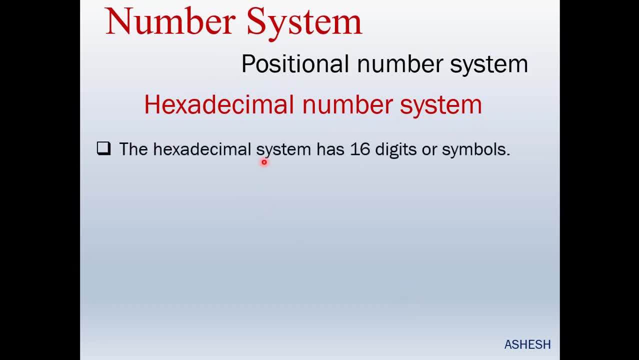